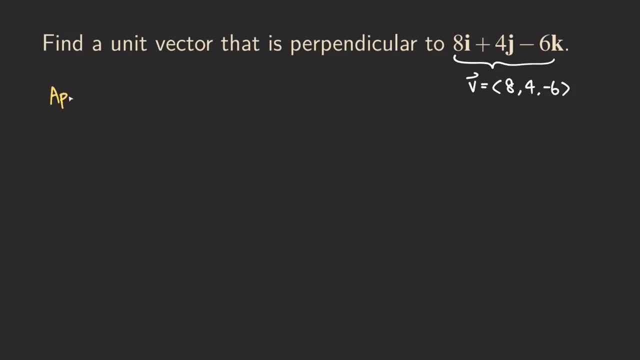 let me write it down. So approach one. so we can actually just start with the first approach right here. Okay, so how do we do this? we can come up with a vector. So let's just call this vector that we're trying to figure out as, as let's say, v1.. Okay, and then we call this ABC, because we 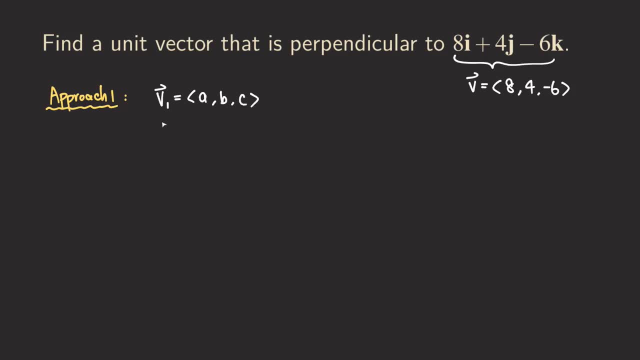 don't know the answer yet, right? So just call them ABC And then. and then what we do is that we are going to take this vector- v1, and then take the dot product of this v, So dot them, right? So what happens is that we are going to just do v1 dotted with v And 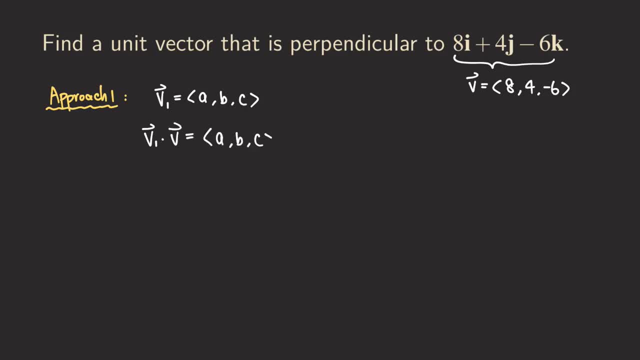 that means we are going to get a and then b and then c, dotted with eight, four and negative six. And if they are perpendicular, then what happens? they're supposed to be giving you a dot product that will be zero, Okay. so what happens is that if you take the dot product you should be, 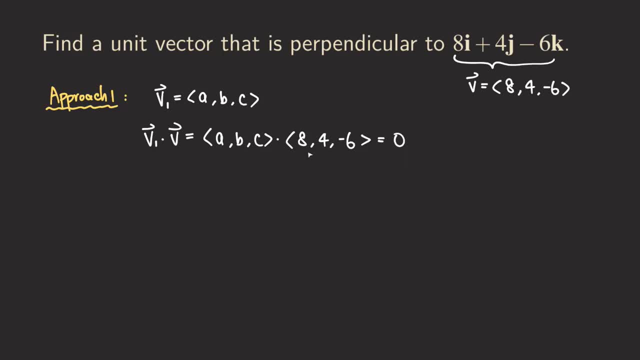 getting zero. So those two vectors that perpendicular to each other. So now what happens is that if you compute this dot product right here, then we are going to get a plus four b, and then minus six c is equal to zero. And so you may say: how do we come up with 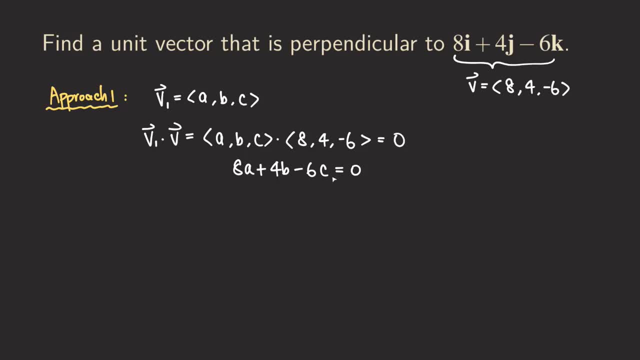 the answer, Because this is a an equation with three unknowns right here And, as I said, it doesn't really, we don't really have like a unique answer here. So that means we can actually just pick some numbers for abc and then just make sure that 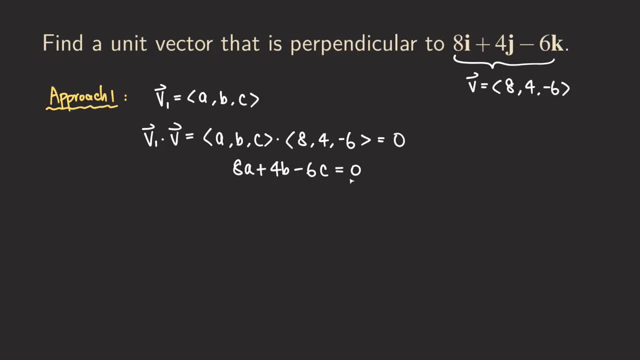 we can find a set of abc that will satisfy this equation. So the easy way to just just to just to look at it is that the eight and four we can just pick. we can pick something like this: Let's say we pick. let's say we pick a to be one and then B to be one. Okay, so that means you're just. 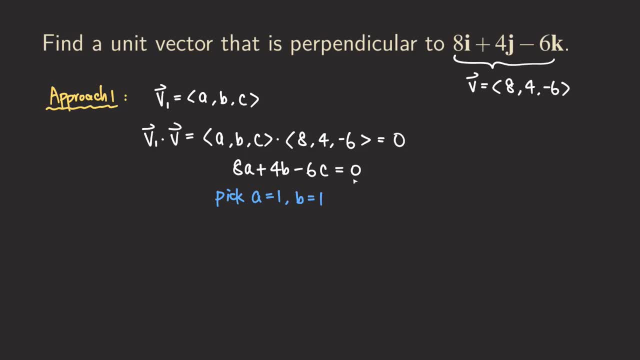 adding the eight and the four, we get 1212 minus six. c is equal to zero. So C must be what, In this case, C in this case. in this case, the C will be what must be two. So we actually come up. 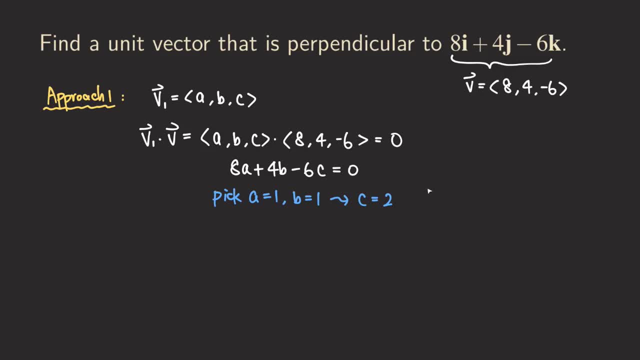 with the answer for v one already, right. So what is v one then? that gives us that v one is actually equal to one, then one and then two. Okay, so that's the vector that is perpendicular to this v here. 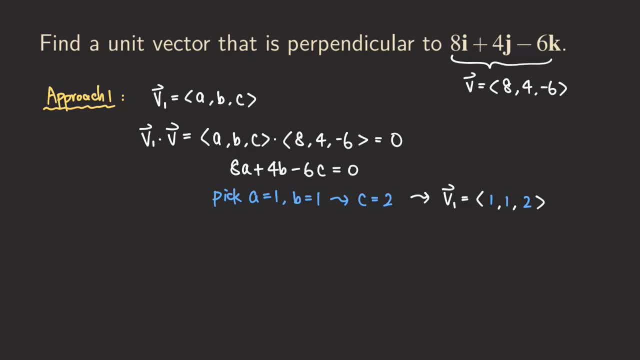 Okay, because it comes from this equation Now, and then you may say what's next. the next step is that we just want to find the unit vector, And that is actually really simple. we just take this vector and then multiply by the reciprocal of its magnitude. So the idea is really simple. So we 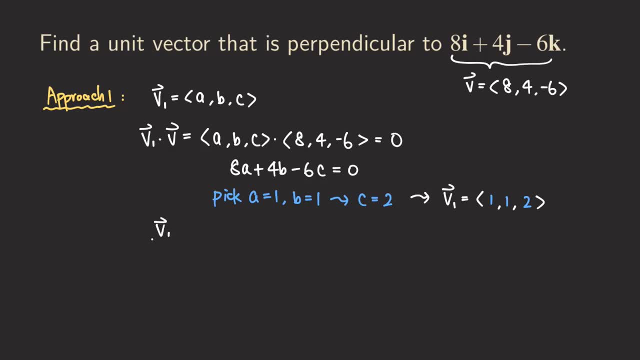 we just find the answer as v one over magnitude of v one, And then we have the answer. So we are going to just get 112.. And then divide by its own magnitude, And so we are going to get one square plus one square plus two square. 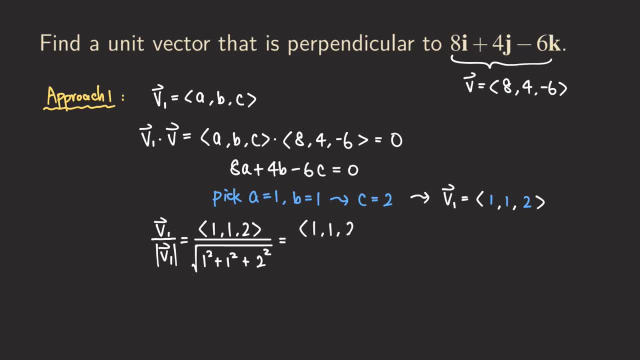 So what do we get here? we are going to get 112.. And then in the denominator, we are going to: let's see, So this is one, this is one, this is four. So we are going to get one plus one plus four. so we 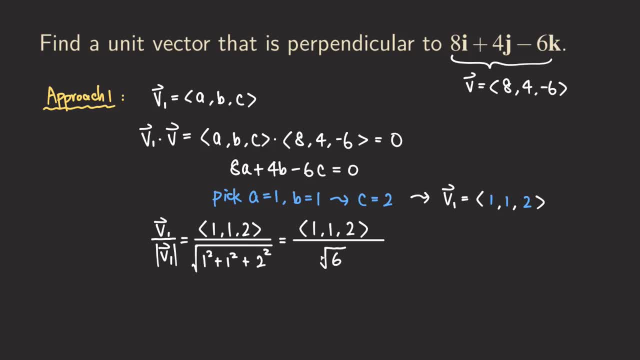 get six. So we get the square root of six as the denominator, and then we can divide by its own magnitude. Now just write down the answer. So one answer that we are getting is one over square root of six, one over square root of six and two over square root of six, And this is a unit vector. Okay, And 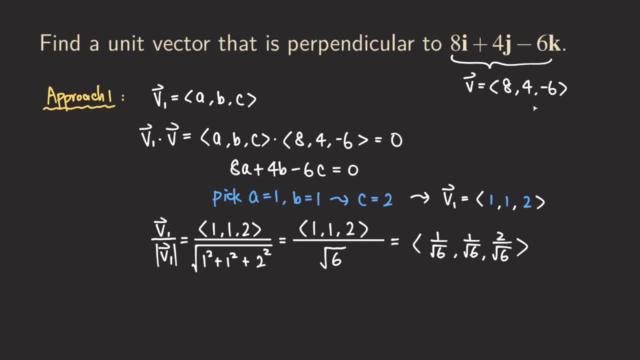 that is also perpendicular to the given vector v. Okay, so that's approach one. that's one way that you can do it. this requires you to just just pick some numbers and then that will satisfy this equation And then you can come up with the answer. And if you don't like that, let's say you. 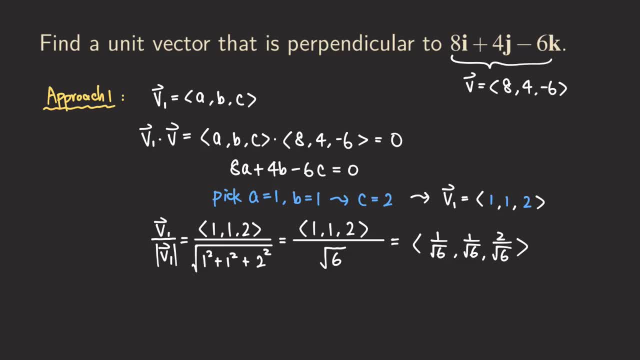 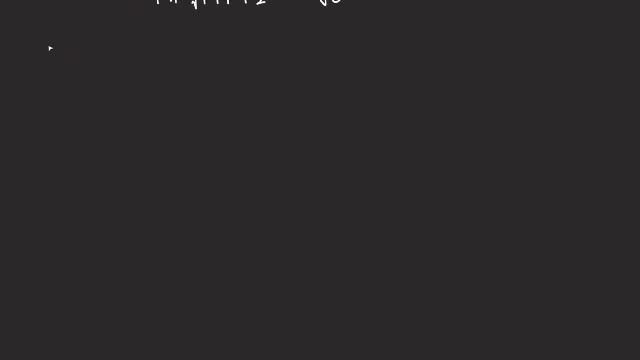 don't feel like picking numbers and here is another way to do it. So what happens is that I'm going to show you a second way to do it, And so right now we are going to just talk about approach two. Okay, and then you may say: how do we do approach to the approach to this? It's to use the. 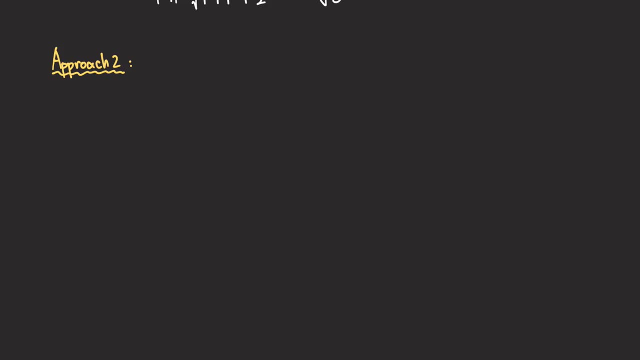 idea for the cross product. And then you may say: why do we suddenly use the cross product? Because when you take the cross product of two vectors, that resulting vector is the cross product of two vectors perpendicular to the vectors that you are crossing. So now, what happens is that then you 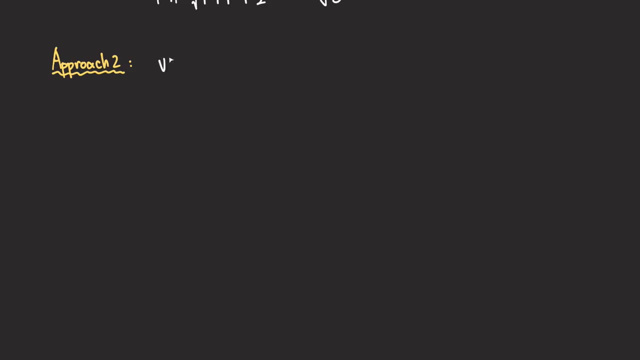 may say: we don't have another vector right, Because we only have the V here. The V is: let's write it down Again: this V is actually just a four negative six. Now you may say: how do we? 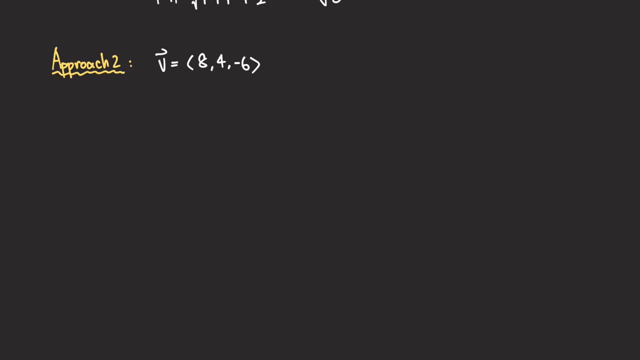 cross the. how do we get a cross product? because we don't have another vector, So we can actually just come up with some random vector here. So when I say random, it actually basically can be anything, but then just make sure that you can. 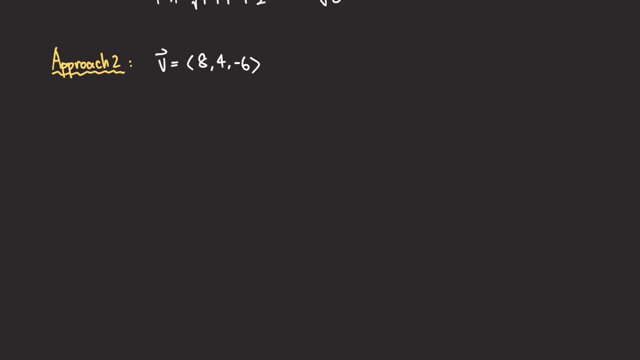 choose the zero vector here. So what we can do, okay, is that we can, we can just pick a random vector. just pick a random, just pick a random vector. what do we have here? we can just call this R, And then what is this vector here? we can just pick the easiest one, we can just pick. I 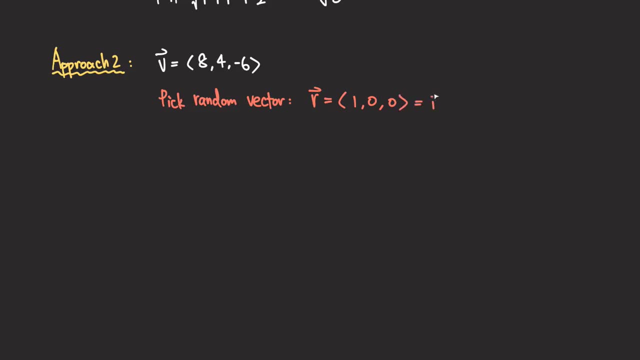 which is 10. Zero, right, so you can just pick the unit vector I okay, and then we just take the cross product of the V and the? I okay. so what happens is that we can just just take the cross product And then. 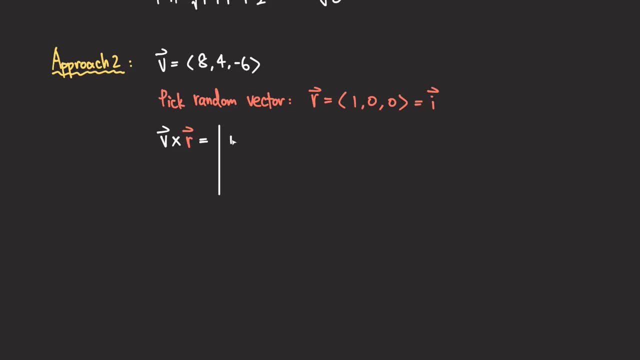 so is what we do? We write them down, so we get eight, four negative six, And then we also have the vector one, zero, zero. Okay, so now what? now just compute right. so we have crossing out the first row. 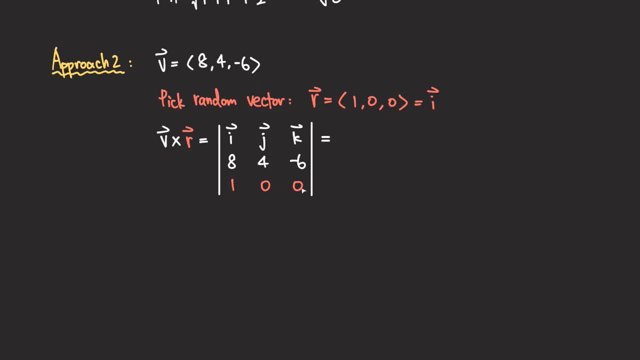 first column, then we are going to get this two by two: the terminal right here, the four times zero, and then zero times six. we just get zero for the first component. So that's easy. Now crossing out the first row and then the middle column, then we are going to get a times zero. 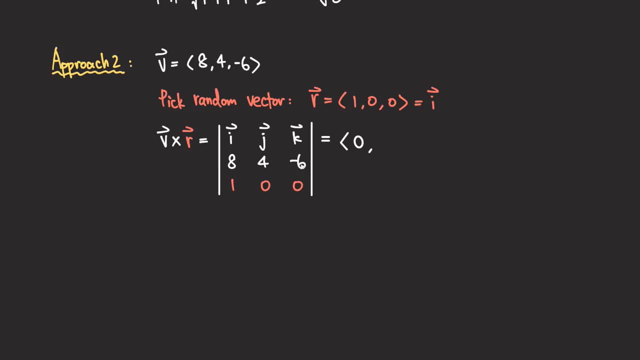 we just get zero and then one times negative six, and then we get negative six. but then we get to subtract this one times a six, right? So we get negative six. and then we get negative six. right, we are going to get positive six here, but then we still get to negate the middle component. 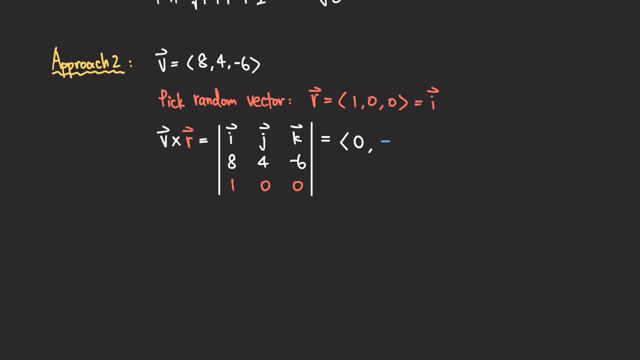 here. So we are going to just get negative six. So we're just going to get a six and then the last component, then crossing out the first row and then the last column, then we are going to get this two by two, the terminal right here. So a times zero is zero. one times four, we get a four. 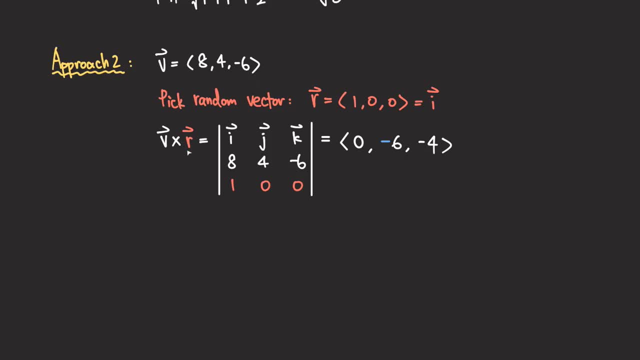 So this is the vector that is perpendicular to both V and R, And actually the R doesn't really, we don't really care about much. we only care if it's this vector, it's perpendicular to this V And in fact it is right. 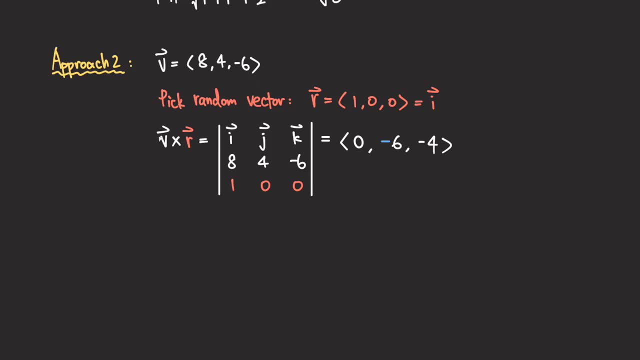 because it's a cross product of V and R, So it's going to be perpendicular to V. And so now we are going to get the vector. Okay, and now what happens is that we can find its magnitude and then divide by its magnitude. then we can actually just get the unit vector that is perpendicular to the V. 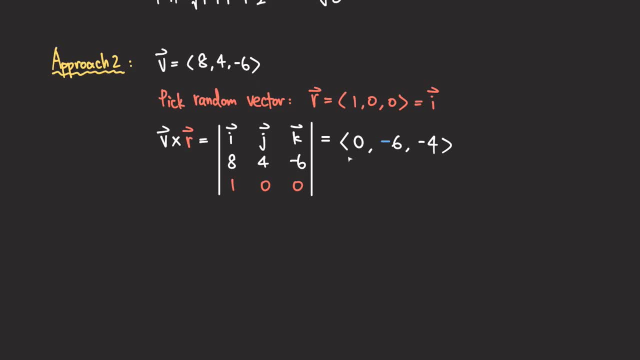 So how do we do it? we can actually call this one, we can actually call this one V two, And then that's another answer that we can get for this problem. So we are going to get V two over V two over the magnitude of V two. So we are going to 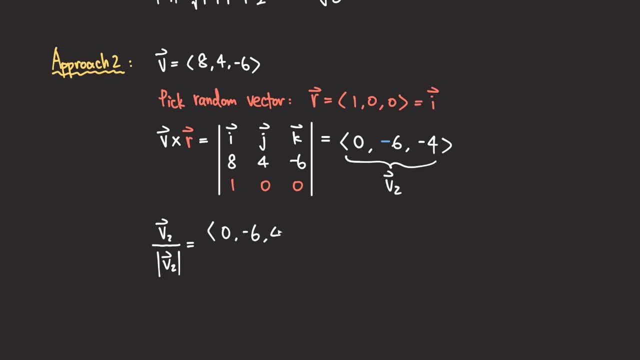 get zero negative six for the numerator, And then the square root of zero square, plus negative six square, And then plus negative four square, And then we are going to be getting what we are going to be getting: zero negative four and then four at the top, So that's stays the same right. And then we are going to be. 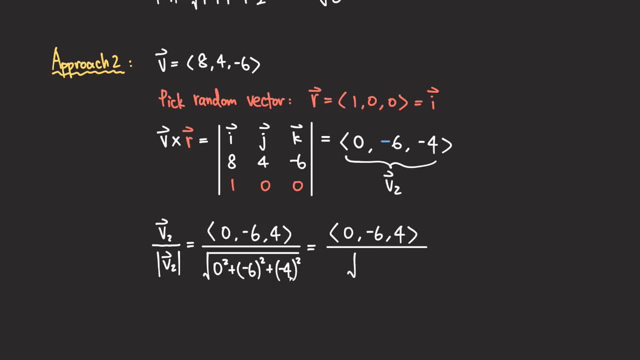 getting. Well, let's see. So this one is 36.. This is well, let's actually just write it down here. So this one is 36. And this one is 16. So, adding the 36 and the 16 together, we are going to get. 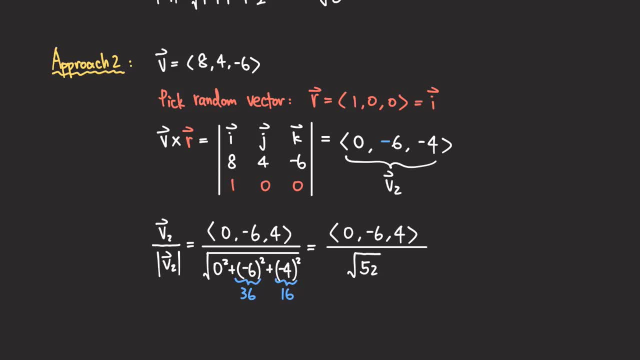 52.. Okay and then so as you know that the 52 can actually be broken as four times 13.. So the four is the perfect square. So you're just going to get a two. So we are going to get zero negative.